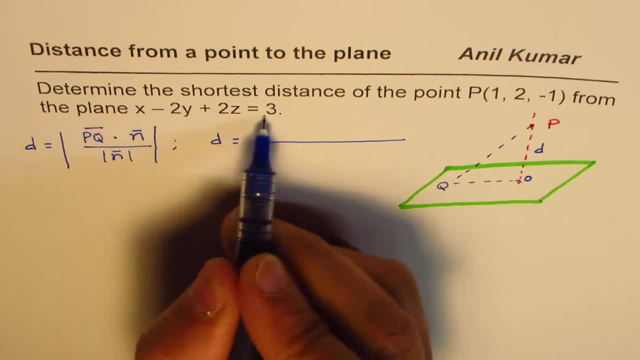 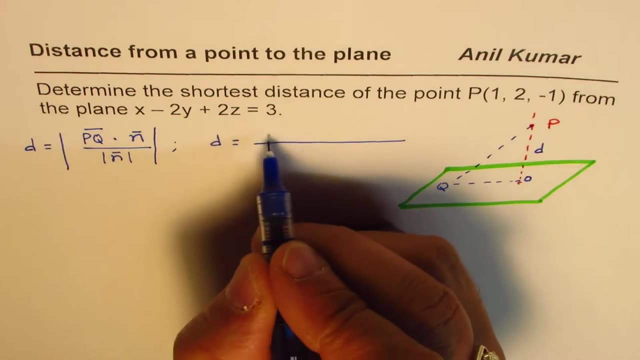 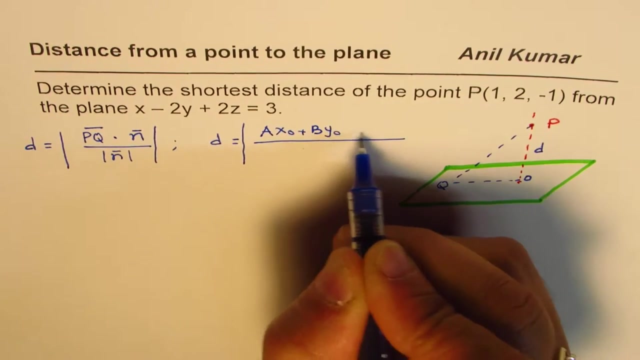 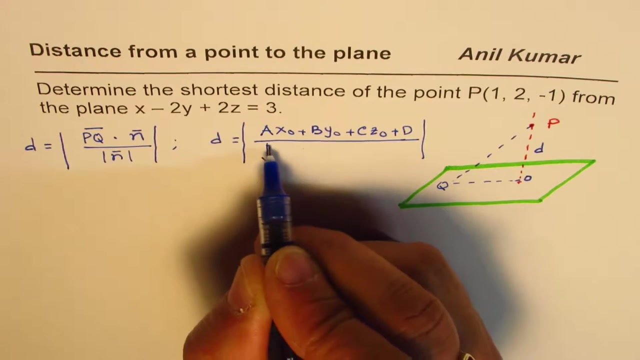 distance is equal to. Whenever the equation is given in, I should say, scalar form or the Cartesian form, then the formula is that the absolute value, of course AX0 plus BY0 plus CZ0 plus D, divided by A square plus B square plus C square, So that is the absolute value, of course, AX0 plus BY0 plus CZ0 plus D. 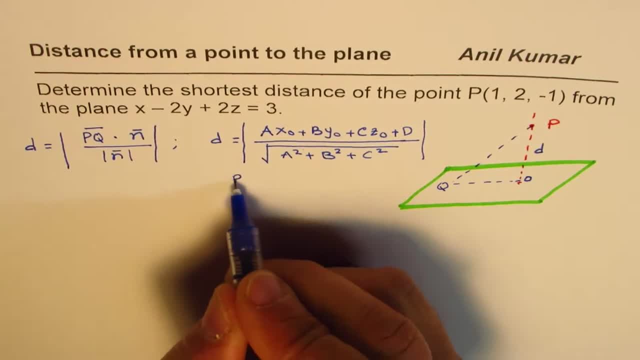 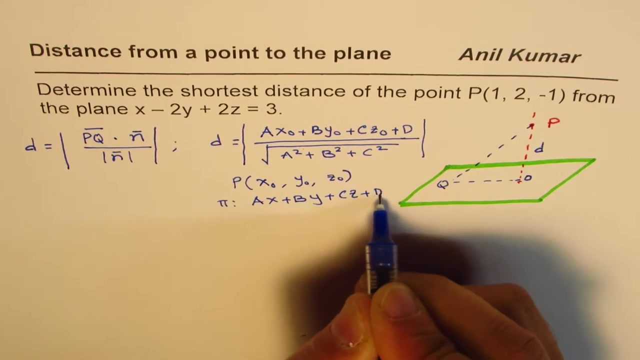 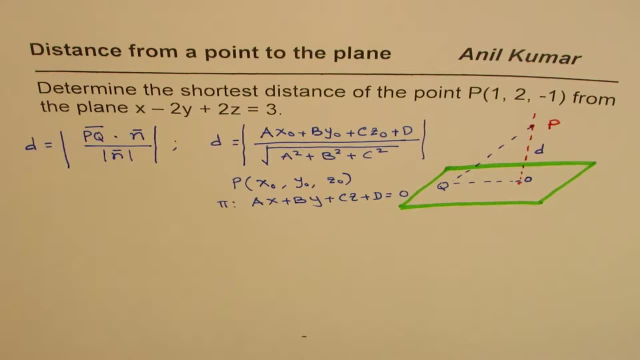 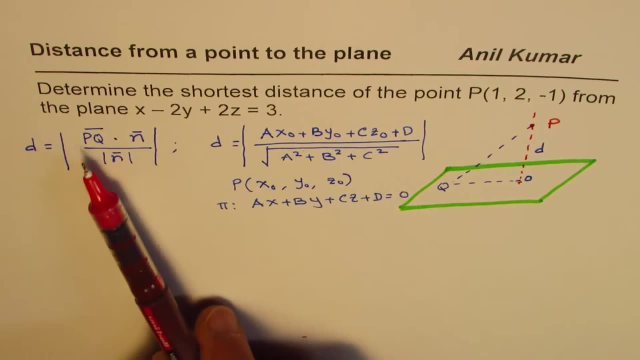 So either of these formulas can be applied to solve such equation. So let's do with both. this is a very straightforward formula which can be applied. Let's start with that Now. to begin with, we need to find we are already given the point P. 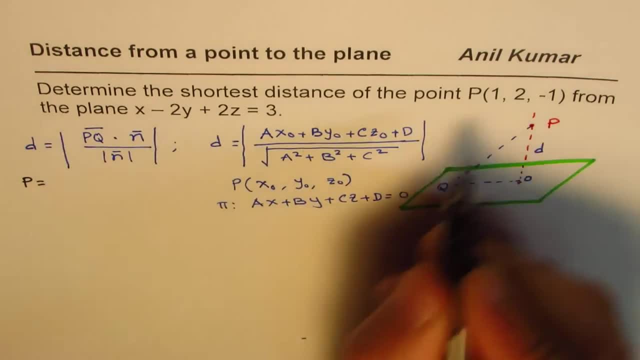 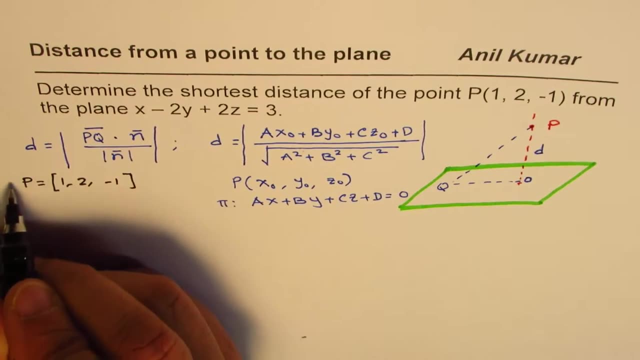 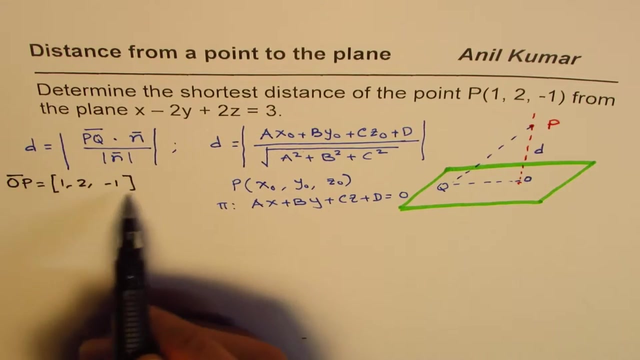 Right, So we are given the point P, which is, which is one 2 minus 1.. Right, So I should say now, when I write like this, let me write vector OP. So from origin, let's say this is our original, So, So from origin, this becomes the position vector. 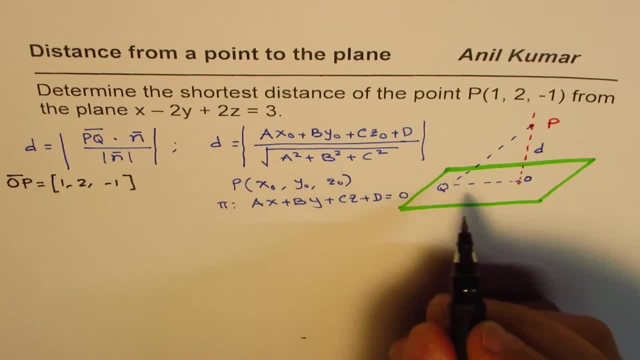 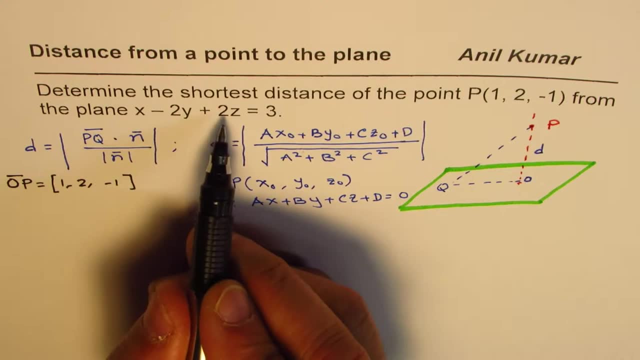 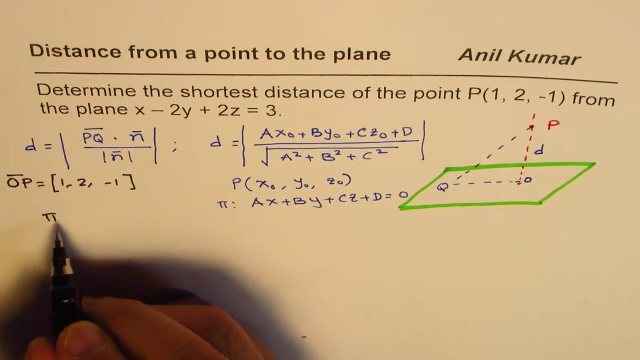 Right Now. let's take a point Q Now to get a point Q- q. we are given the plane so we can select some convenient values for x, y and z to find x right. so so what we are given here is a plane. we normally write plane with symbols like pi, let. 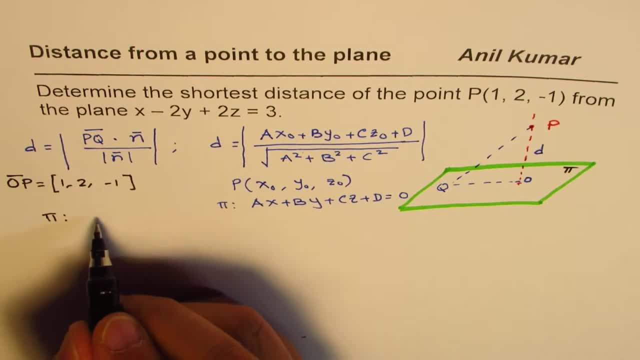 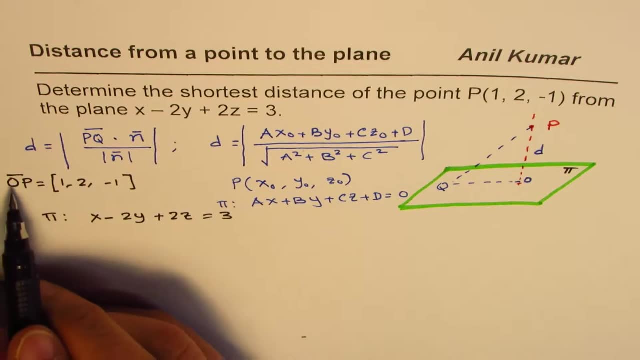 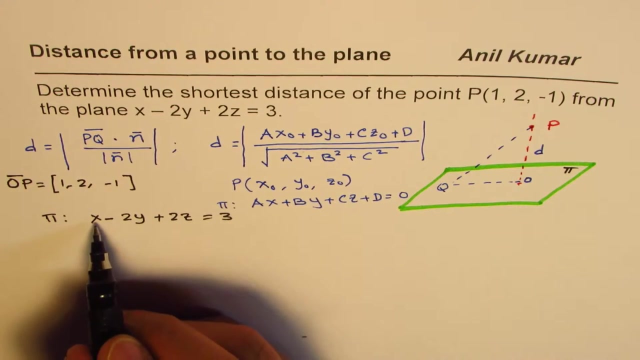 me write here pi, okay, and the equation of plane is: x minus 2y plus 2z equals to 3. so to find a point q, we can select values. so if i select y and z as 0, i get x as 3 to get an idea. so so the point. 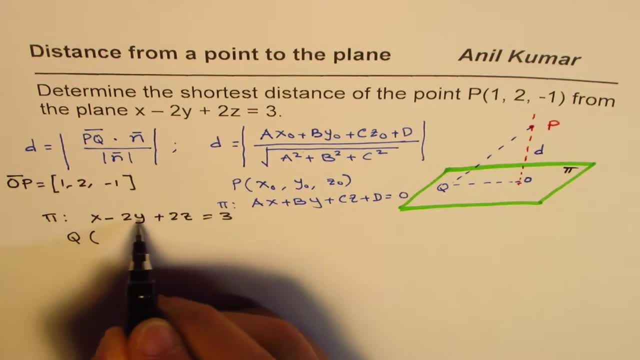 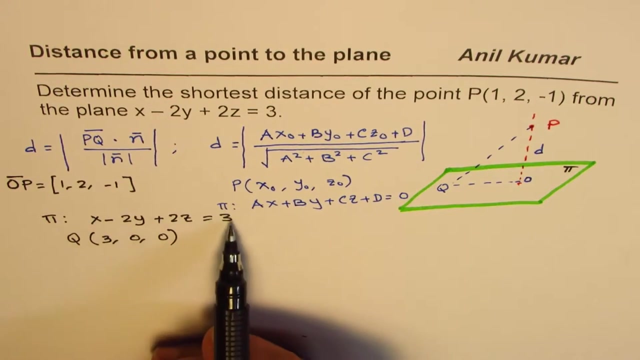 q could be. i'm selecting these as zeros, right? so just for easy calculations. so i could write this as 3, 0, 0, right so? so i've selected a point q, only for convenience. you could set at any point, since it satisfies this equation, it lies on the plane. that's the whole concept: 0, 0. so we get x equals to 3, correct? now the, the. 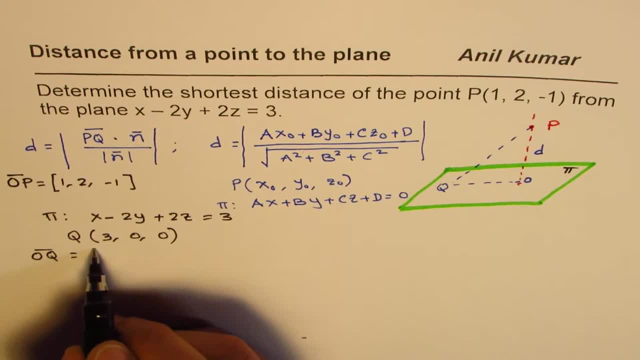 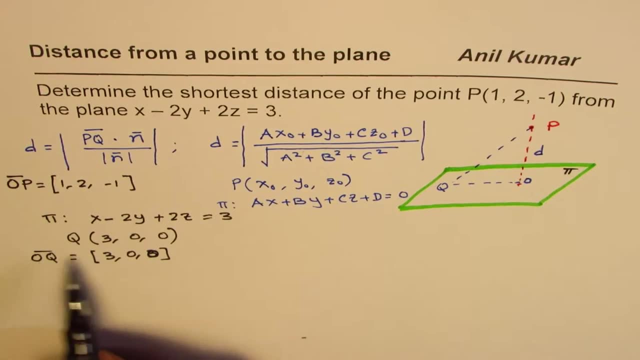 vector oq will be written like this: right, so right, it's correct. i mean, okay, so we have this vector oq, so now what is what is pq? so pq will be oq minus op, correct? so i'm just taking time to do all this so that all understand what we're trying to do, so that 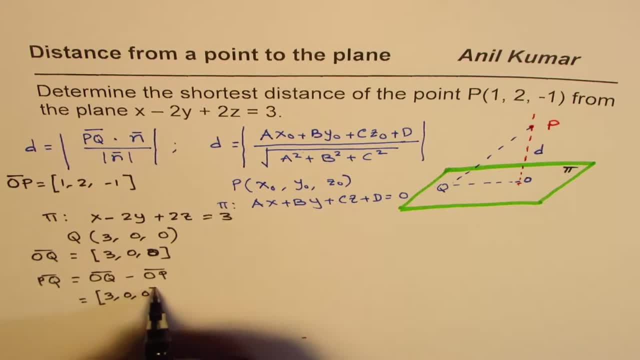 means it is 3, 0, 0. take away 1, 2 minus 1, correct, and that gives you 3. take away 1 is 2 and this. take away that minus 2 and 1, so that becomes pq. now we'll apply the formula and get the result. 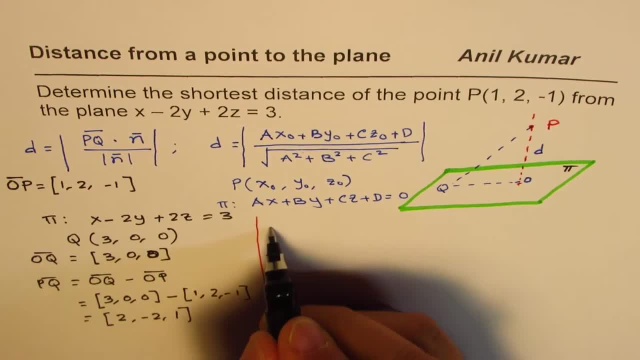 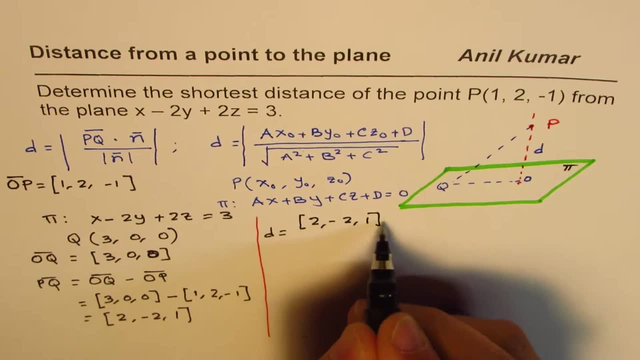 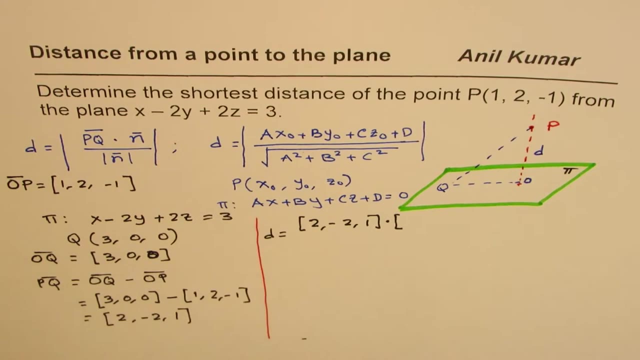 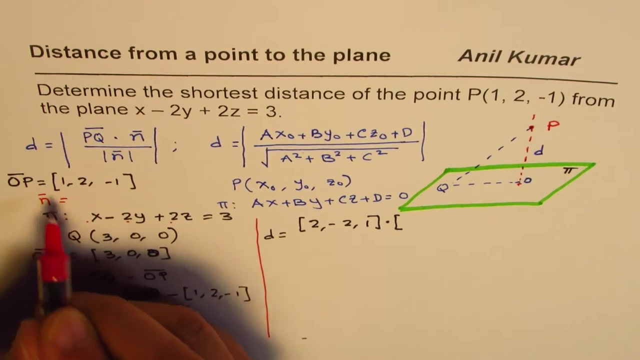 okay, so pq. so distance d is equals to pq, which is 2 minus 2. 1 dot n for us is- you can read normal from this equation, from the plane. so when you are given the plane here, these coefficients give you the n value. so let me write n as equal to 1 minus 2, 2 right, so i'm just taking time to do all this. 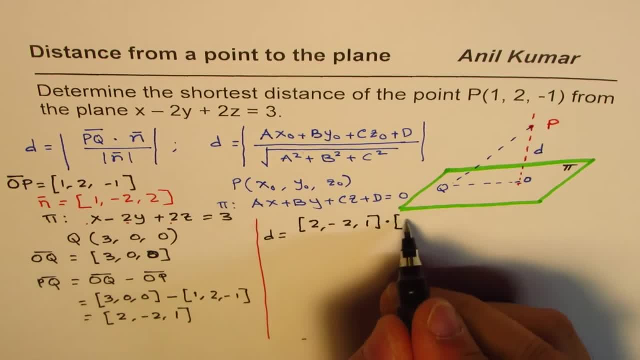 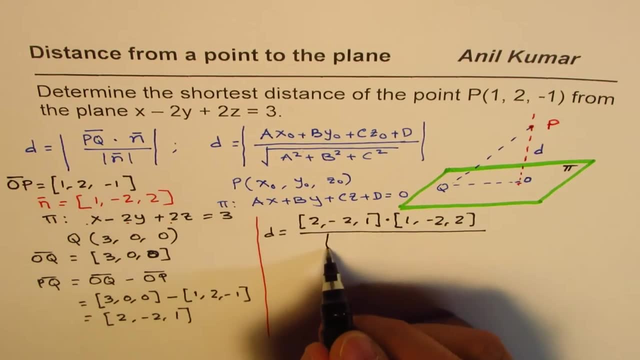 so that is the value of n. so n is 1 minus 2. 2, that is the dot product divided by the magnitude. so 1 square plus minus 2 square plus 2 square square root, now that is equals to 2 times 1 is 2 absolute. 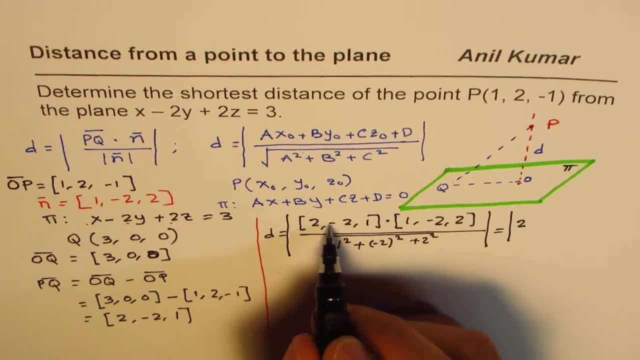 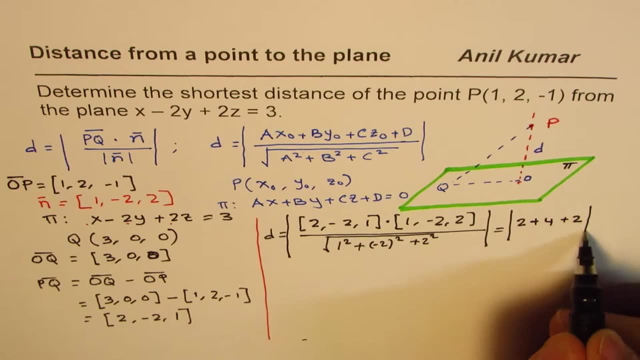 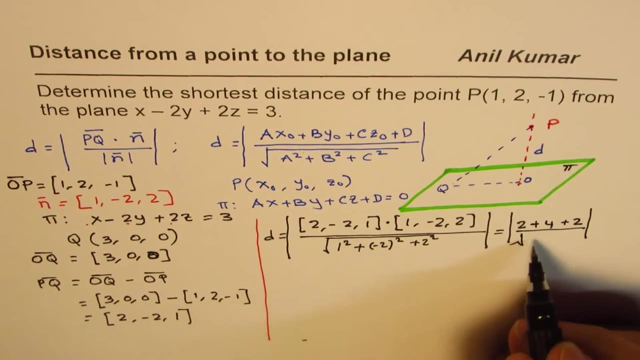 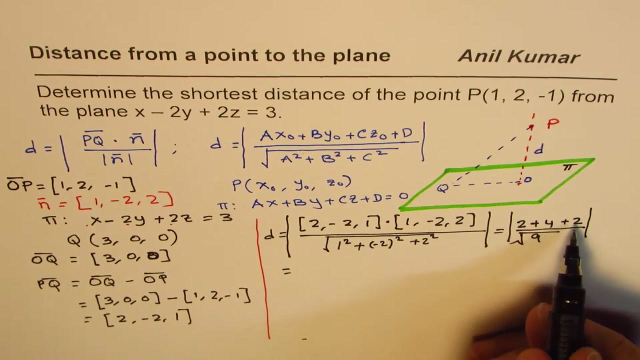 value great. minus 1 times minus 2 is plus 4. 1 times 2 is plus 2. right absolute value divided by square root of 1 plus 4 plus 4, that is square root of 9, and this gives you 2 plus 4, 6 plus 2, 8. square root of 9 is 3, so you get 8 over 3 as the 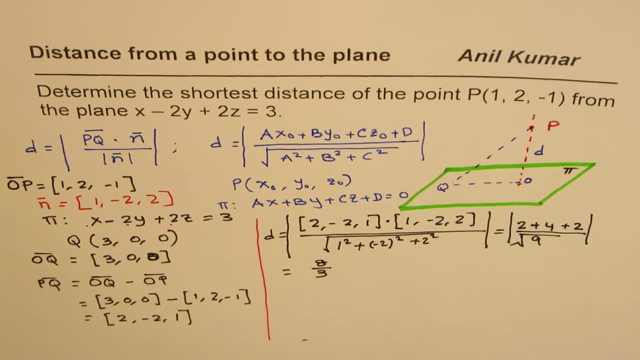 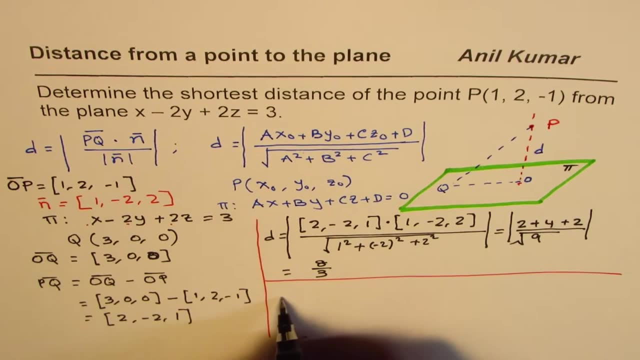 distance correct. so that is how you can find the distance. now let's do the alternate way of finding the distance: applying the formula straight away. so you found this. that's the right answer. okay, but it takes kind of time, especially when you know this right. so d equals to absolute value. we'll substitute. 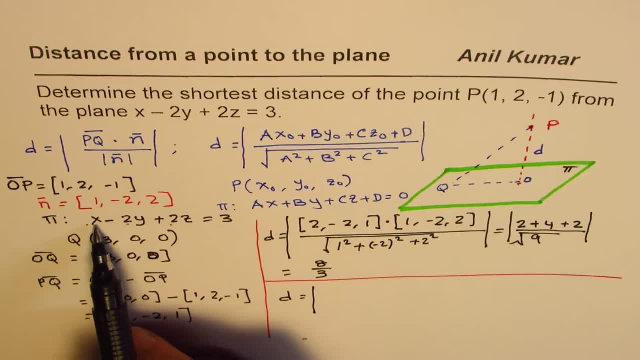 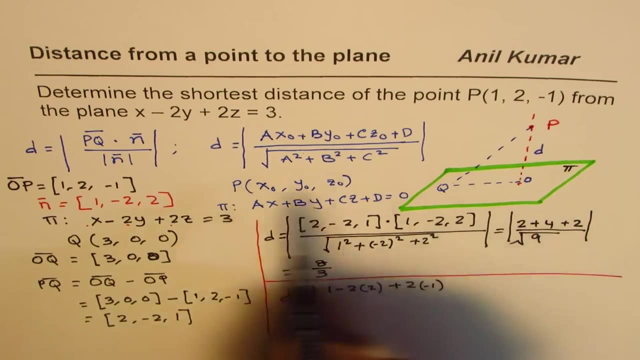 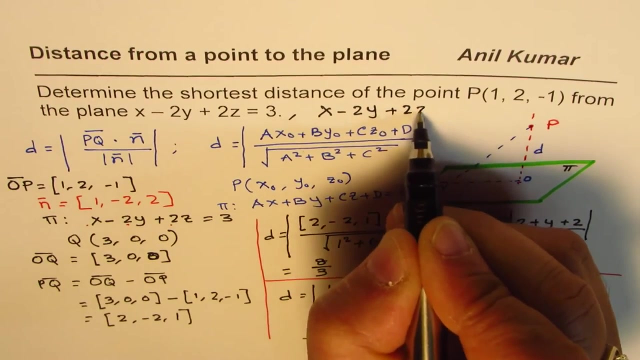 the given point, p, 1, 2, 3 in this equation 1 for x. so we have 1 minus 2 times 2, right, and then we have plus 2 z. z is minus 1 and we'll bring 3 to this side. so i should write this equation as: x minus 2, y plus 2, z minus 3. 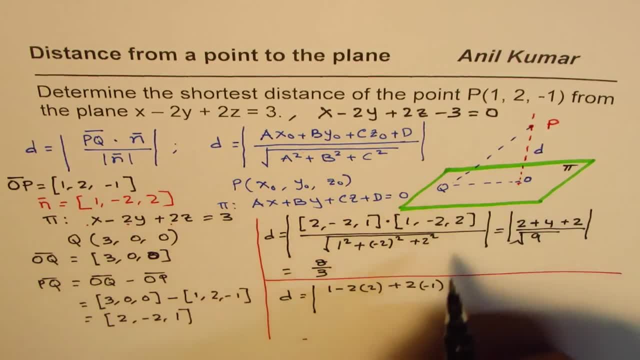 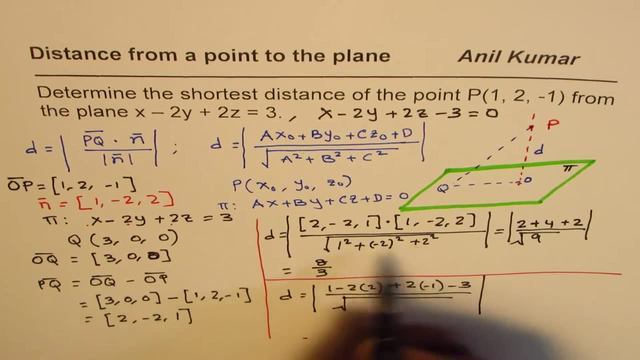 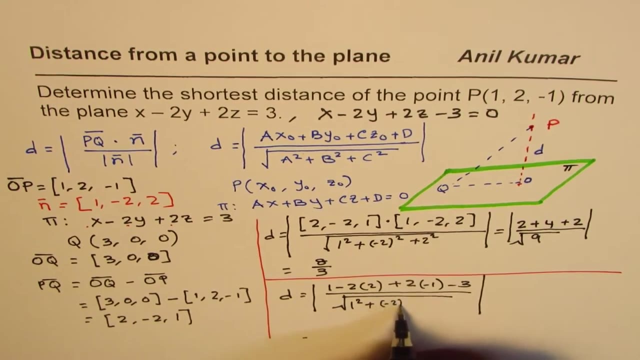 equals to 0, right? so so we get this. and minus 3 divided by square root of same thing, right? that is the same: a square, b square, c square, which is actually the normal right. so 1 square plus minus 2 square plus 2 square, and that gives you. 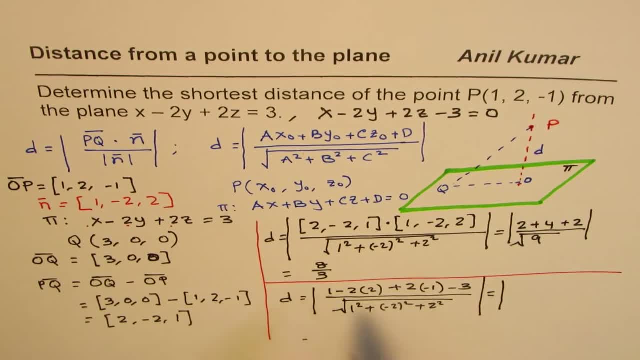 1. 2 times 2 is 4 minus 4, and 2 times minus 1 is minus 2, and this is minus 3 divided by square root of 9. so that is, in the negatives, we get 4 plus 2, 6. 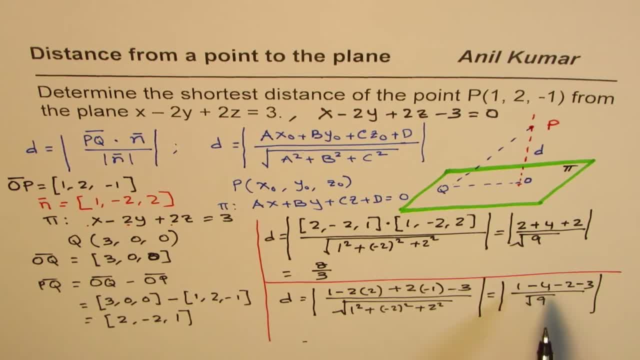 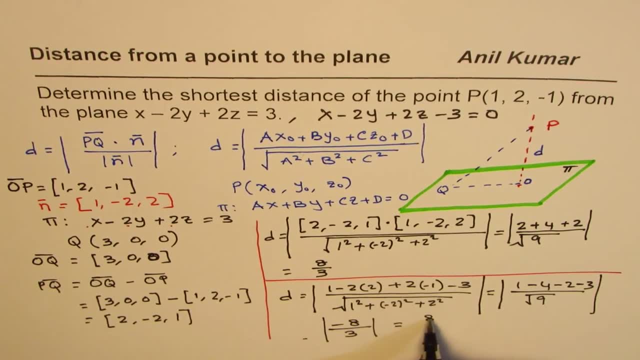 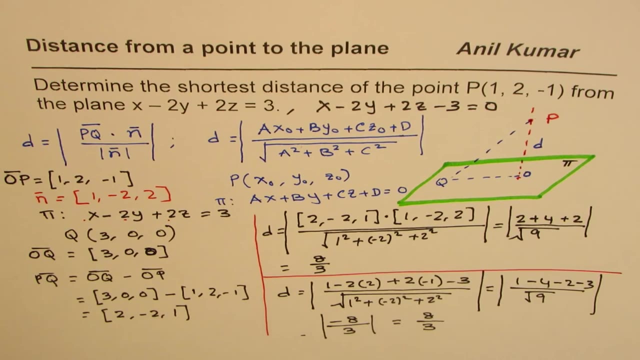 minus 3, i mean 9 and 1. so we get minus 8 over 3 absolute value, and that is equals to 8 over 3. do you see that? so, so you get exactly the same answer. so the application of formula is much better, uh, in some cases. so you should accordingly.